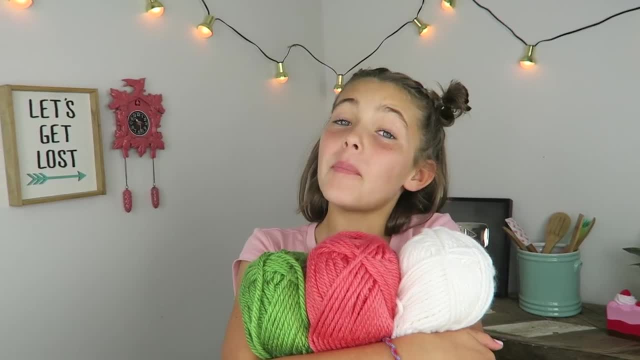 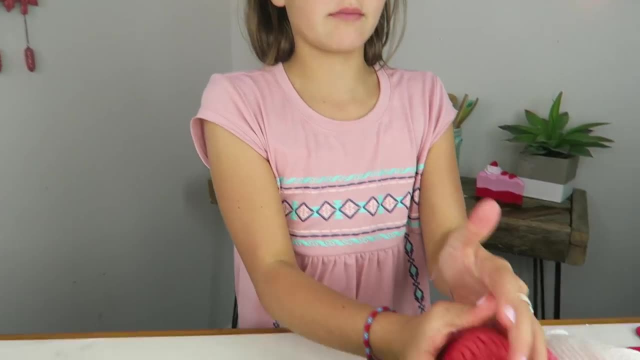 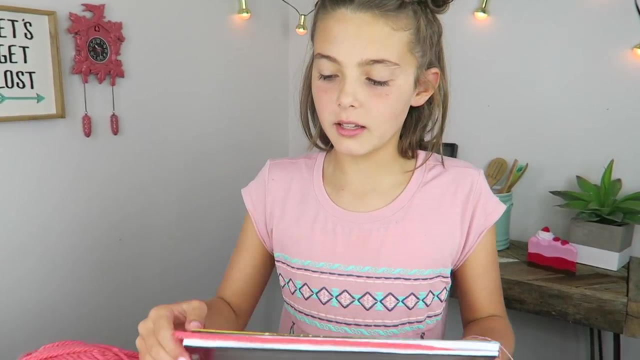 They remind me of watermelon. So we're going to make pom poms and tassels. So first I'm going to teach you how to make a tassel, So pick your color. I'm going to do pink, Okay, grab a notebook and then just lay your yarn onto the notebook like this: 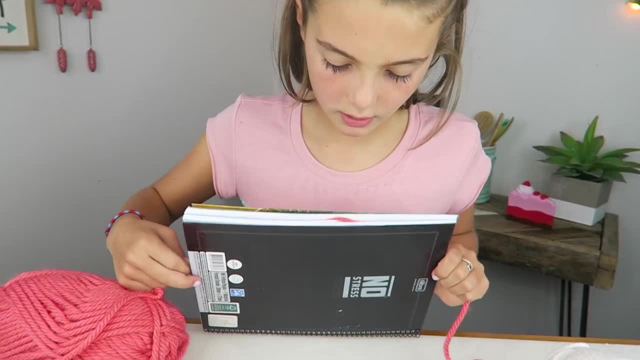 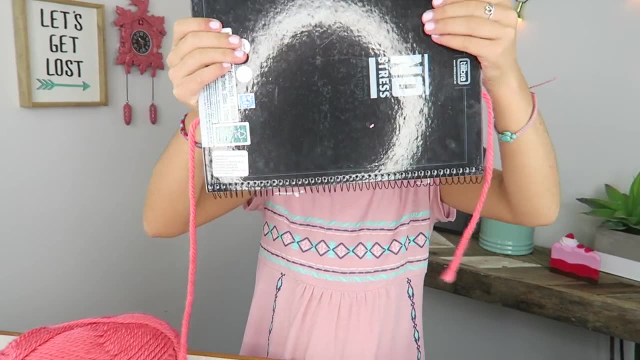 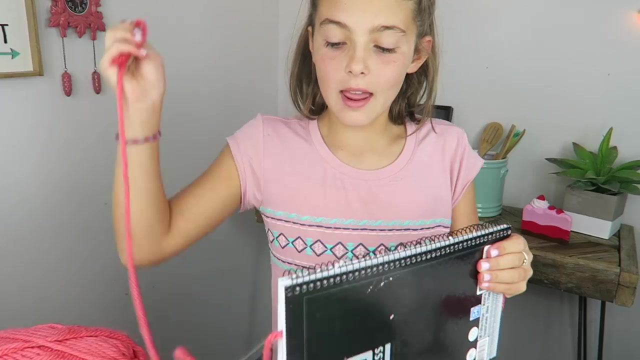 And then stick it into the pages so that it won't move. And then cut, cut. See how this piece of yarn is trapped inside of the book. We're going to leave it right there and move on to the next step. So grab your yarn and start wrapping it around your notebook over and over again. 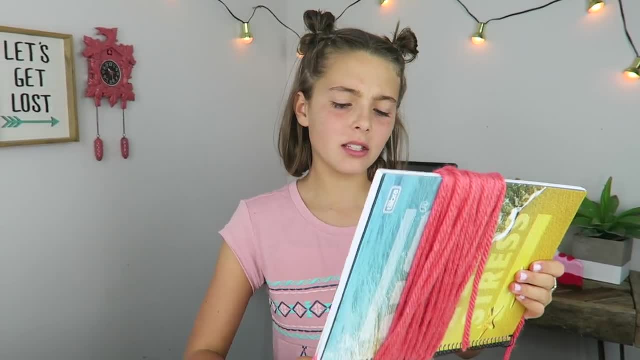 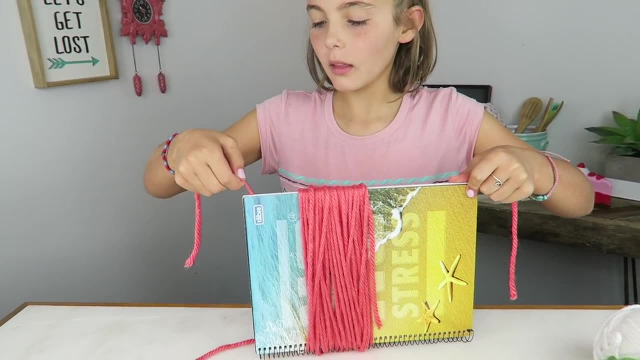 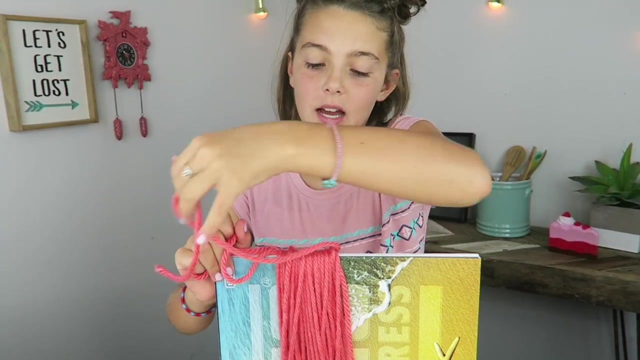 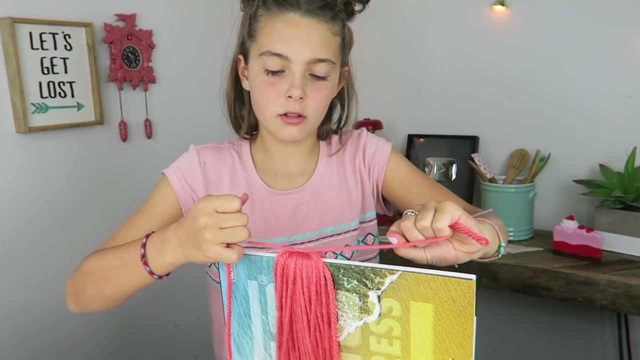 Okay, I think we're good. I wrapped the string around like about 40 times, So now get your string that's stuck in your notebook and pull it up. Okay, and then make a knot. I like to use square knots just because they're super easy and they're super strong. 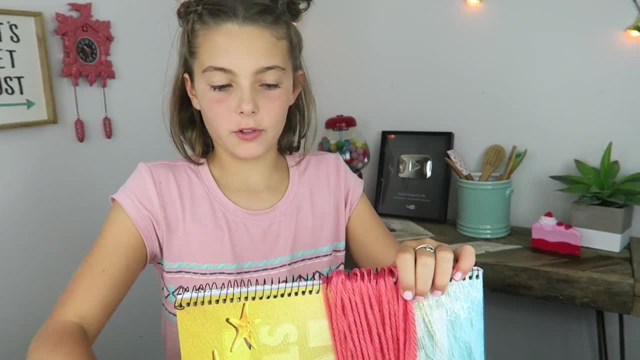 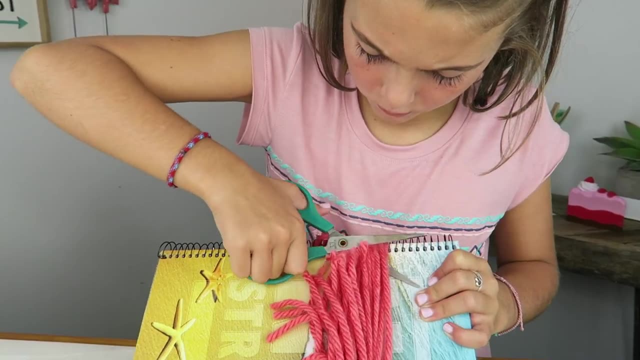 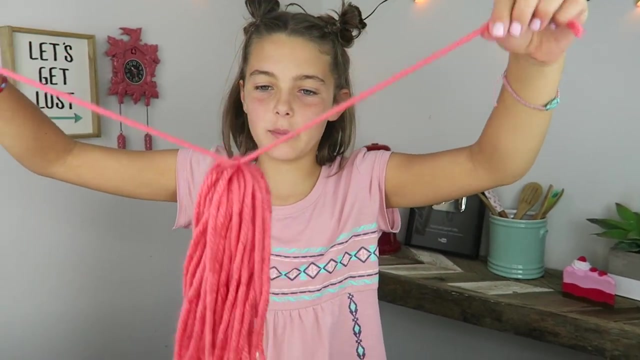 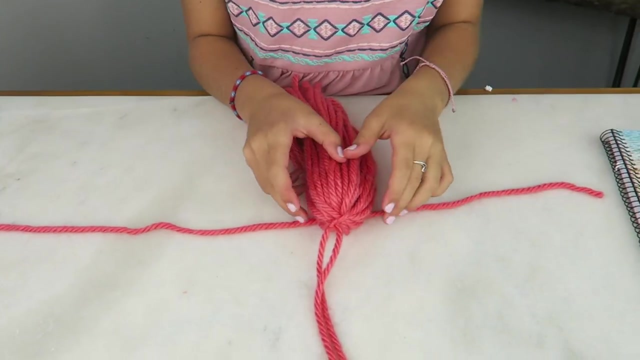 There we go. Now you're going to go to the bottom of your notebook and start cutting it. It looks like an octopus. Now we're going to secure it with another string right at the top. Lay your tassel right on there. 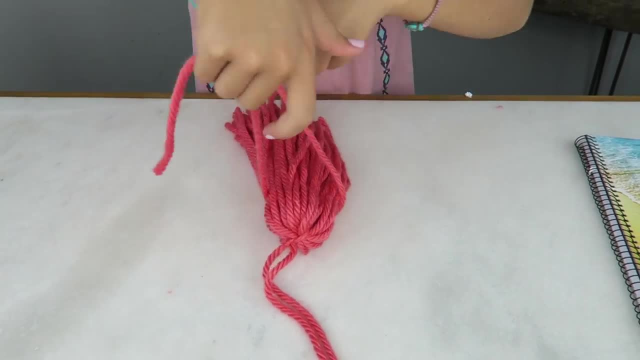 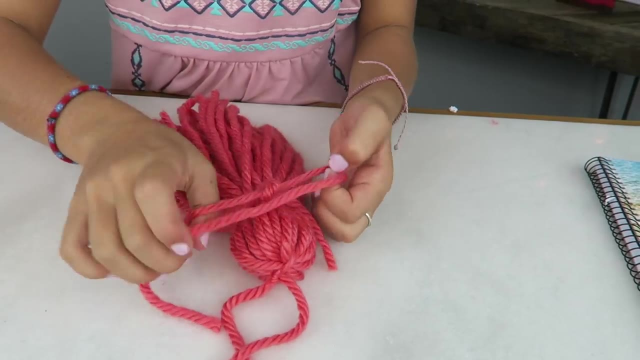 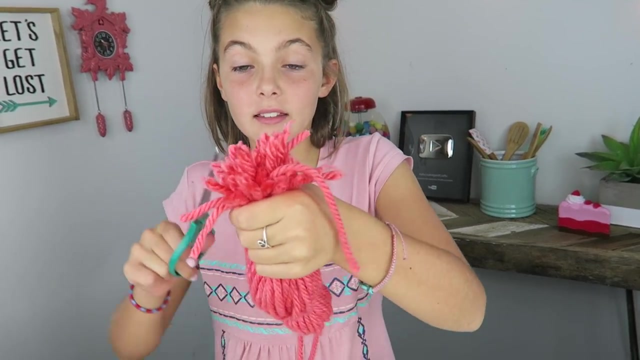 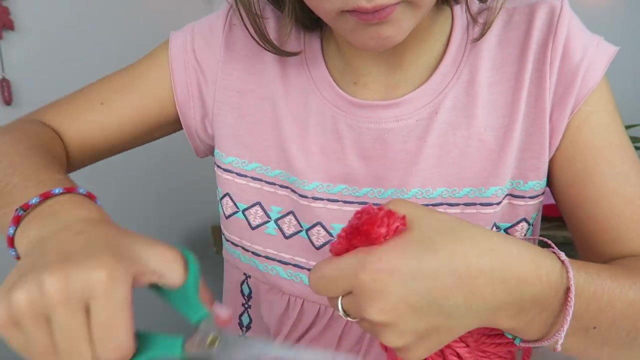 Make sure you leave a little bit of space at the top There. Okay, now we're just going to trim it. All of these strings are different lengths, so we're going to make them all even See how it's nice, and even at the top. 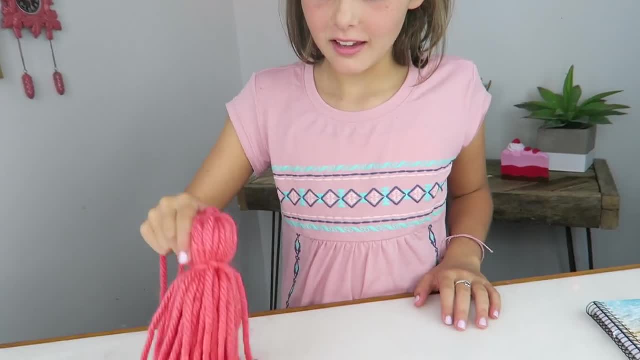 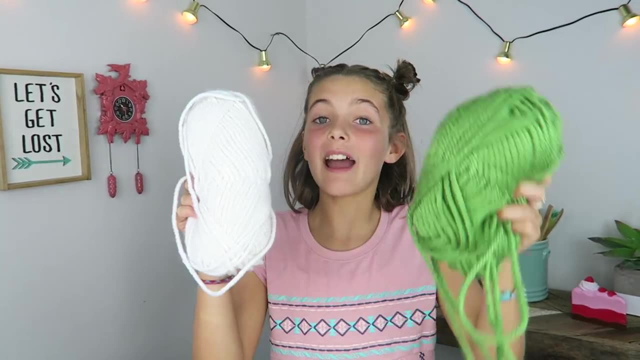 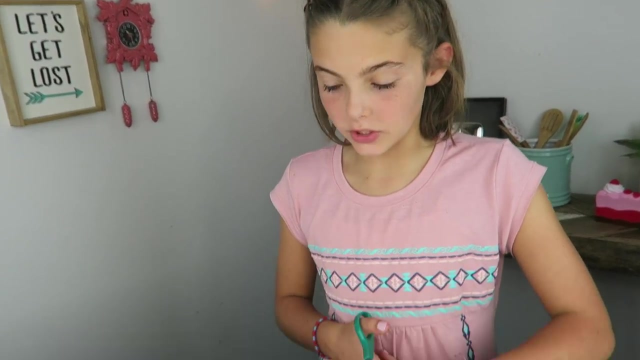 I could play with this forever. It can also be used as a broom. See On to our pom poms. We're going to use white and green. For this one, you need a hair pick and white string. We're going to cut a long piece of string. 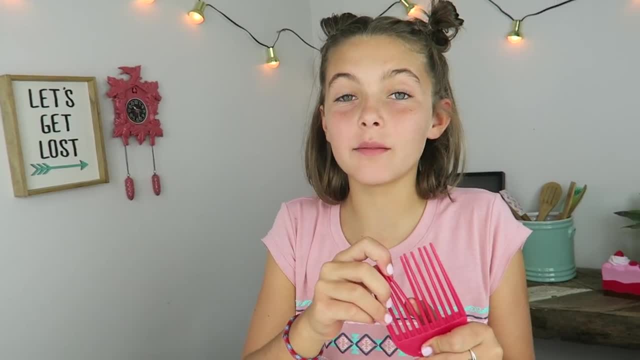 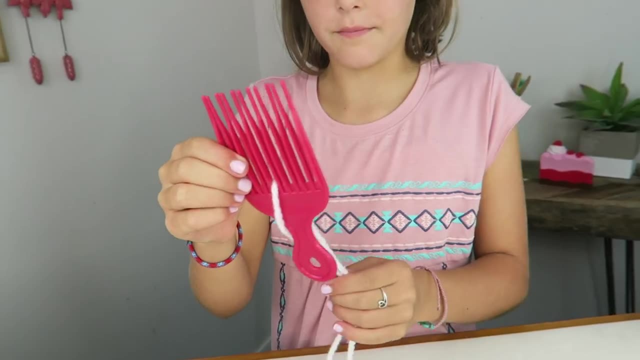 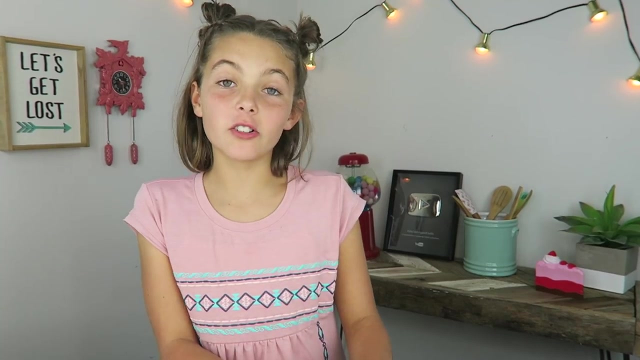 Okay, I'm just going to put it right in the middle of the pick, Right there. Now I'm going to get some other string and wrap it around the pick. I'm going to go around 25 times. All right, I think this looks pretty good. 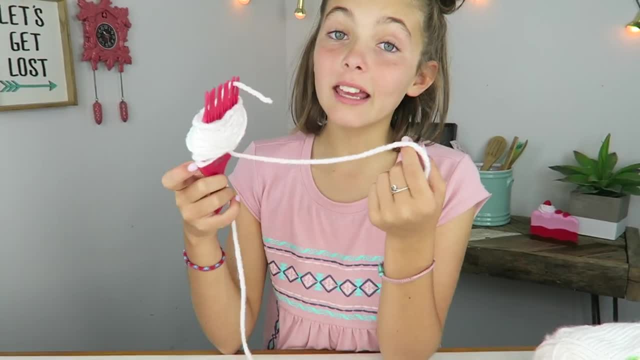 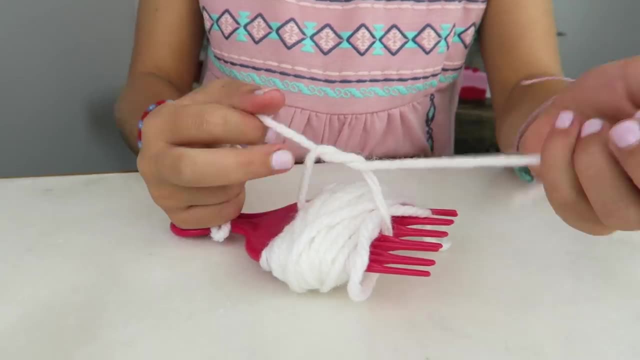 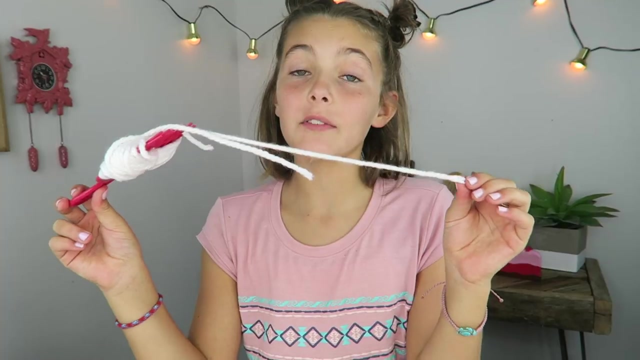 Now we're going to get the string that we put on first and bring it over and tie a knot, And we don't want to cut this off, We want to leave it long so we can attach it to the mermaid blanket. Now we're going to start making the other string. 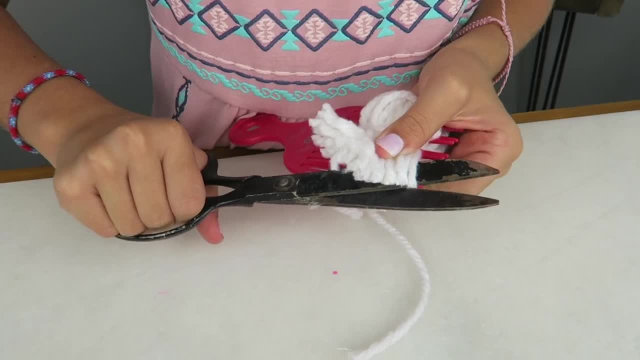 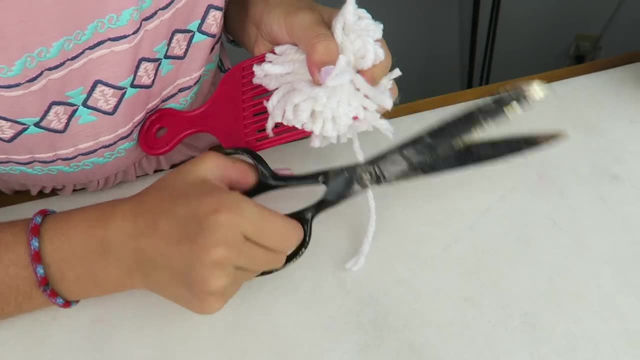 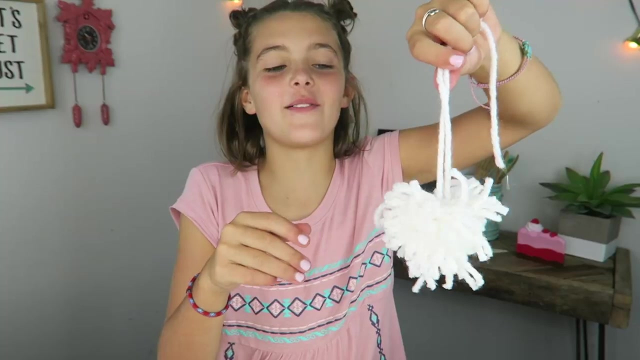 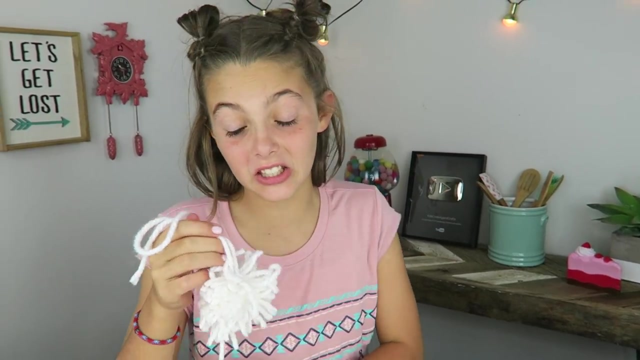 Now we're going to start cutting off the edges. There's one side: Oh boy, There we go. Take the pom pom off And there You have an alien pom pom. No, but seriously, We're going to even the strings out so it looks nice and cute. 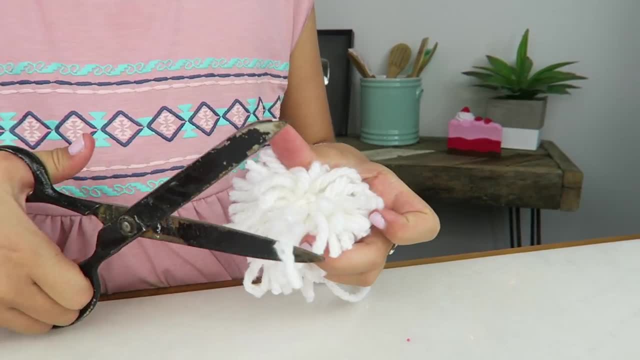 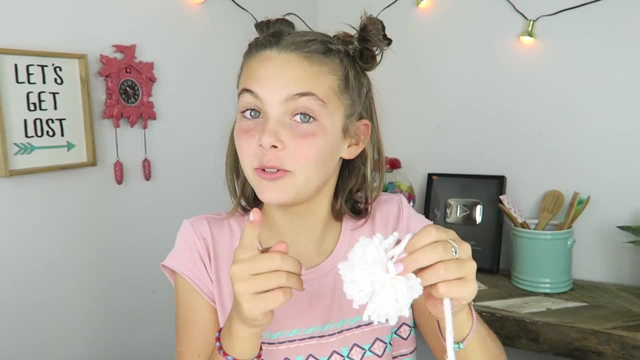 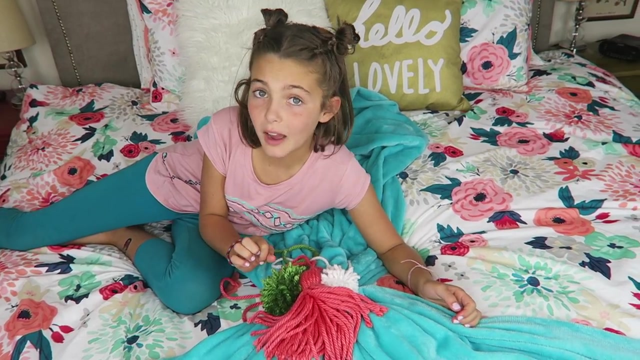 It's like giving a little dog a haircut. There you go, See how it's nice and flat around the edges. That's what you want. Let's go attach these pom poms and a tassel to our mermaid tail. I'm trying to decide how I want it to look. 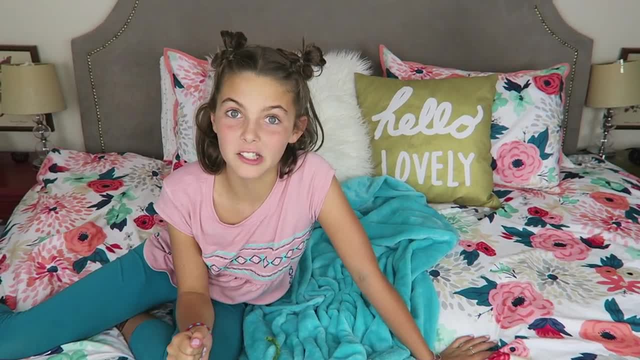 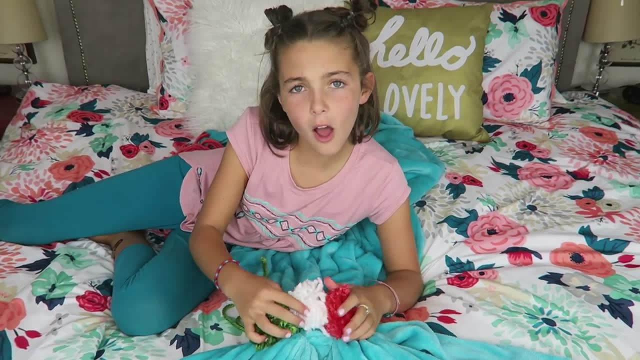 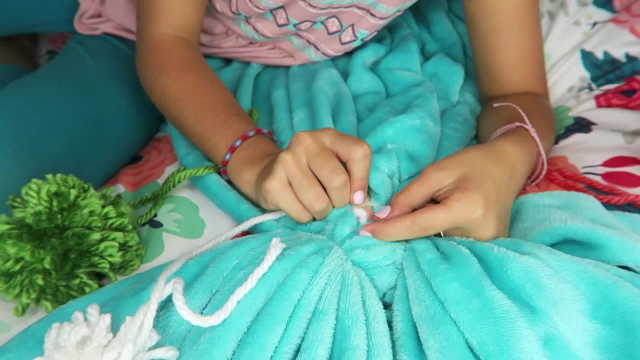 The tassel isn't really working for me, So I'm going to make another pom pom. Wow, This is a perfect pom pom. So I'm just going to put all three pom poms across, Just like that. So I'm going to get the string and poke it underneath the zip tie. 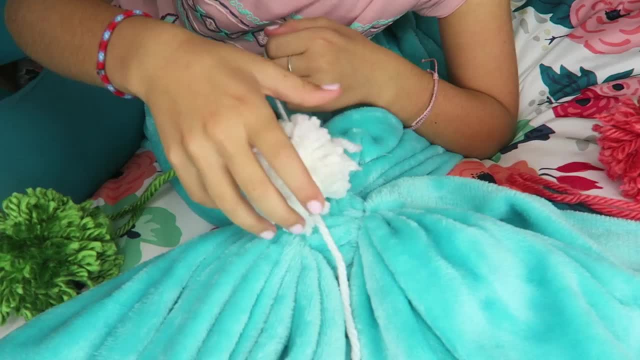 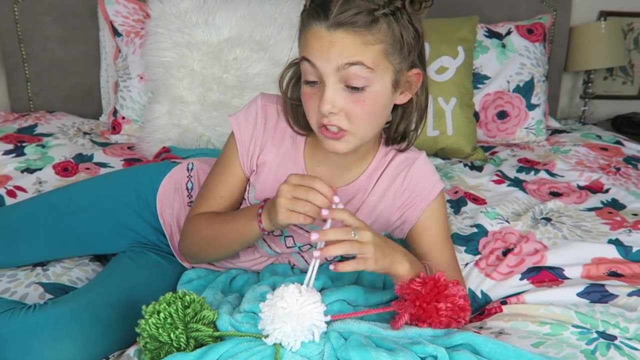 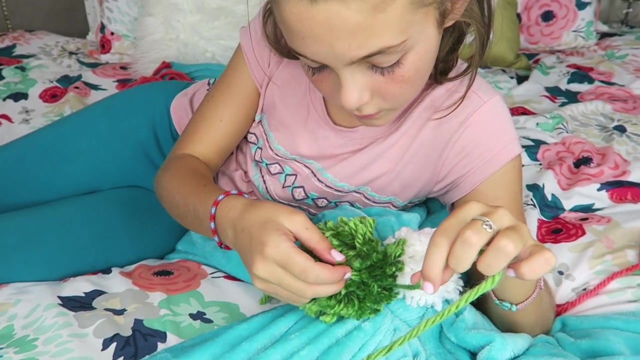 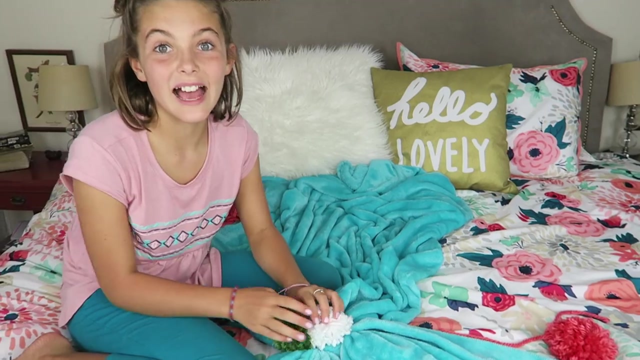 Just like that And pull it nice and tight And then you just tie it on. Okay, there, Now we're going to cut off the remainder of the string, So it matches the length of the rest of the pom pom. Last one: